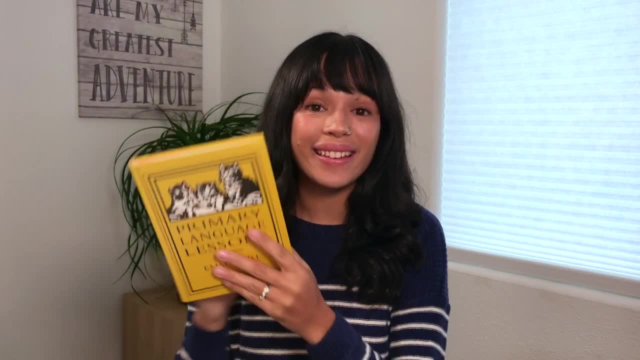 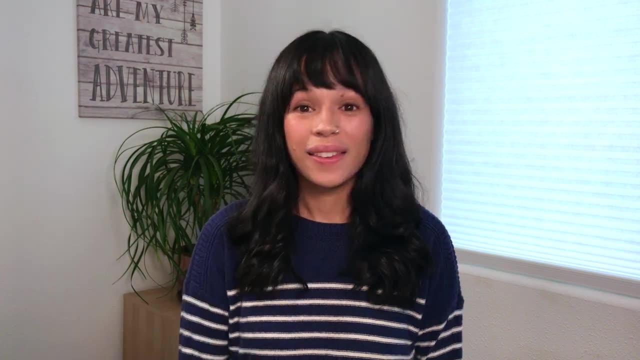 you will see, these days The book is really tiny so it's easy to store. It includes excerpts from classic poetry and it has pieces of classic artwork in it. Since this isn't a modern language arts curriculum, you will most likely want to refer to the Suggestions to Teachers section at 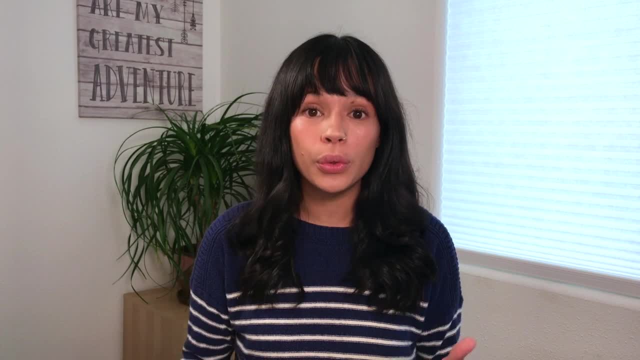 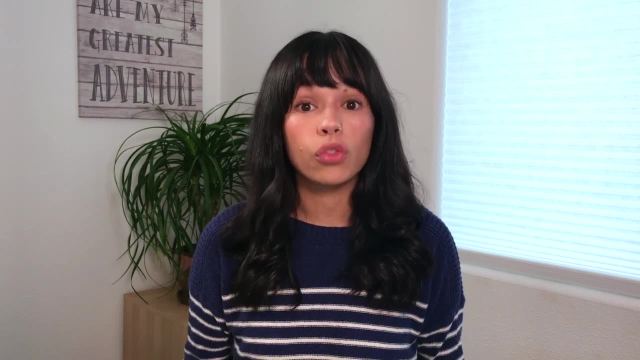 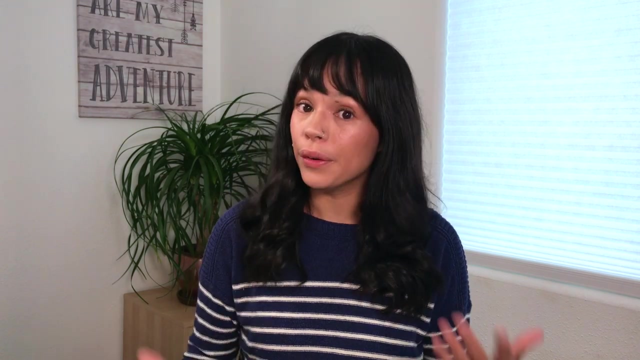 the very beginning of the book, just to know how to do these exercises in your homeschool. So the way that Primary Language Lessons works is it consists of a series of drills. So these are different lessons that teach your kids different language arts concepts. All of these concepts kind of build on each other. so that you can learn a little bit more about the language arts curriculum. So the way that Primary Language Lessons works is it consists of a series of drills, So these are different lessons that teach your kids different language arts concepts. All of these concepts, kind. 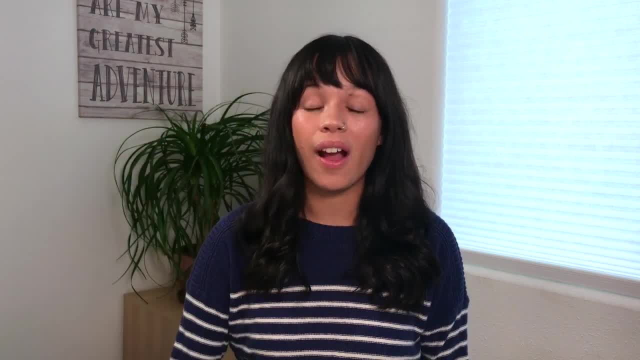 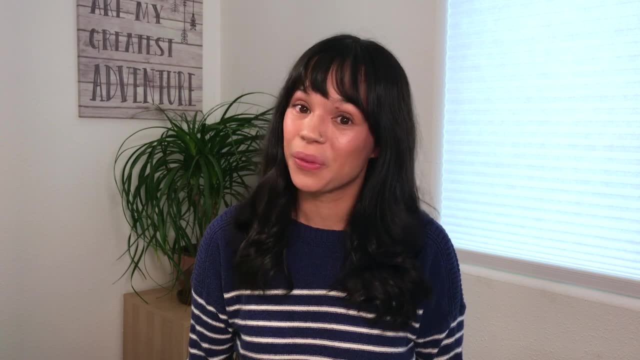 of build on each other so that you can learn a little bit more about the language arts curriculum. By the end of this book, you will be working on writing longer passages, reading longer passages and even doing things like writing letters, which is really cool to me. 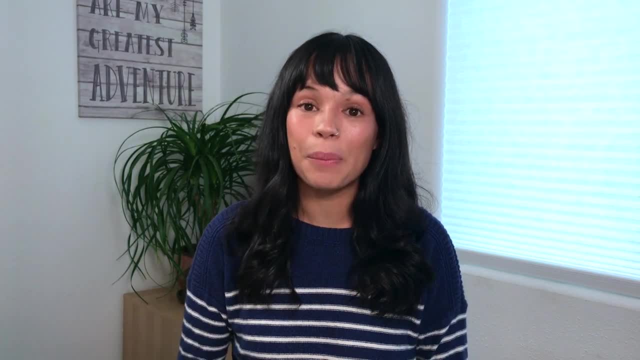 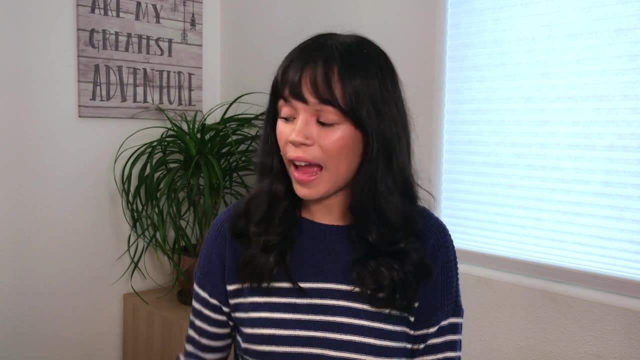 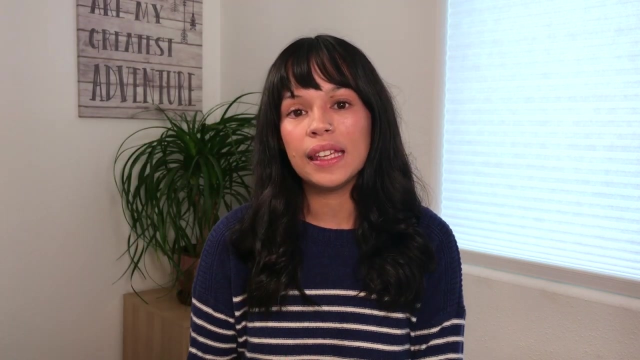 Now I'm going to go over a list of some of the drills that this book incorporates and how I do them in my homeschool. A big one in this book is copywork. For copywork- I actually have my daughter in a separate notebook that accompanies the textbook- write the sentences given. 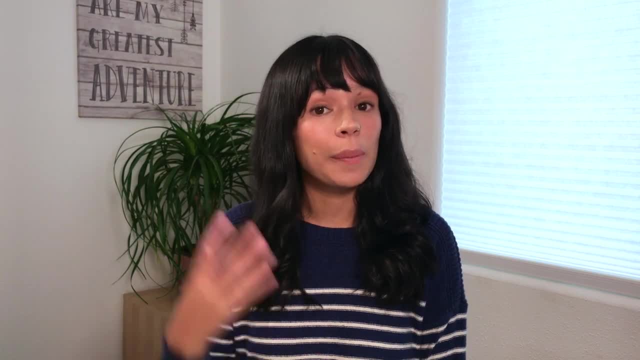 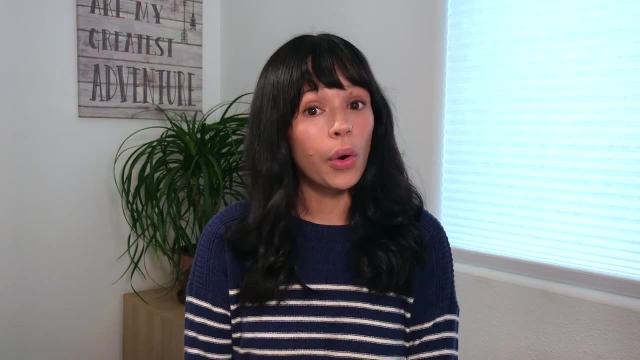 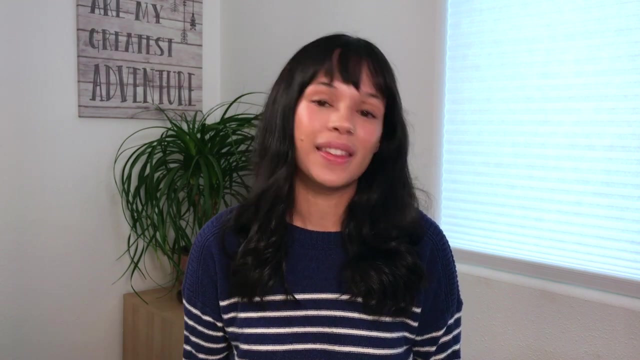 based on what she sees in the textbook. This is not done from hearing the sentence. It's not done from memory. It's done from actually reading the sentence and copying exactly what they see For memorization. this requires reading a poem to your kids and having them memorize the different 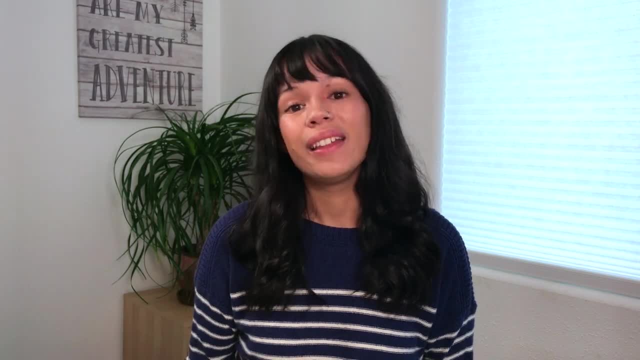 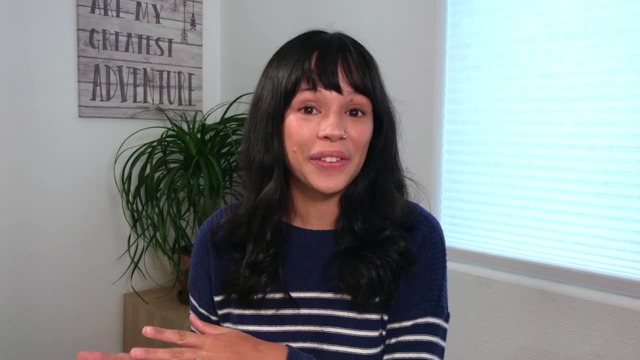 sections of the poem every day. For this exercise in the book it does sometimes take us almost a week sometimes to get the poem memorized. In order to move on to the next exercises in the book, the poem needs to be completely memorized. At least that's how I do it in my homeschool. 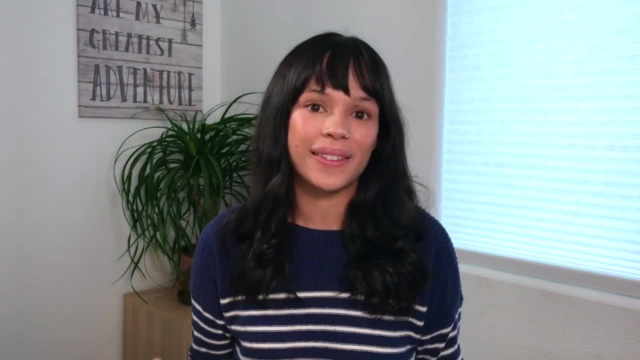 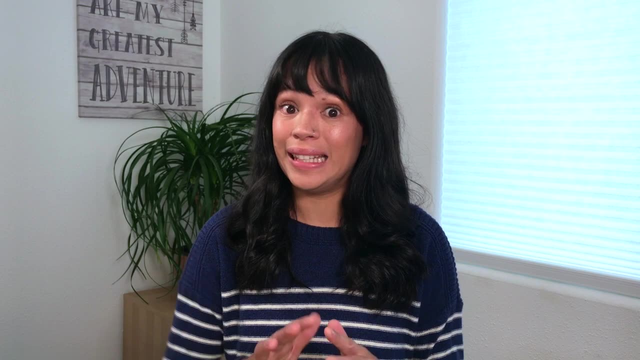 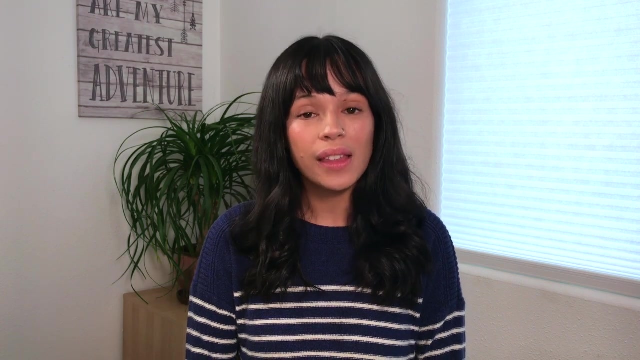 This really does build the skill of memorization and recitation for poetry. Another skill similar to copywork is dictation. This is one that I kind of didn't have any experience with, so I referred to the suggestions to teachers section. at the very beginning It said to read aloud a sentence once, just once, and then have your child write. 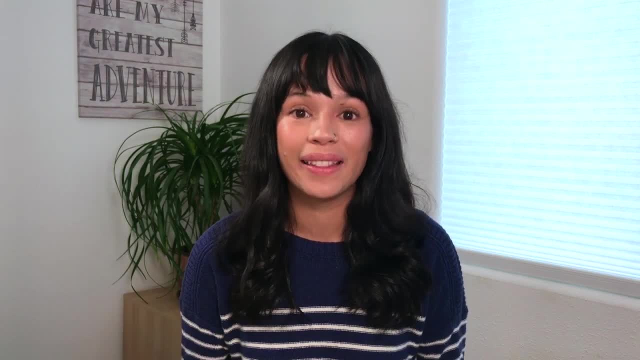 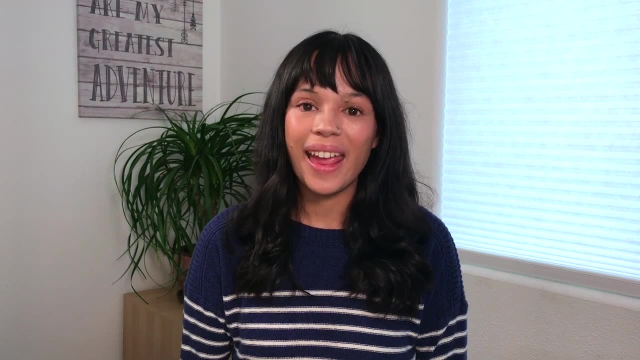 the sentence based on what they memorized from what you said In that one reading of the sentence. the child must write the sentence exactly as read and any mistakes in that sentence do need to be corrected. The way that we have been doing this is. I will do. 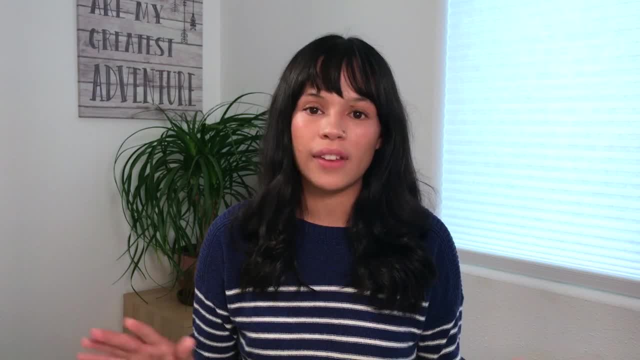 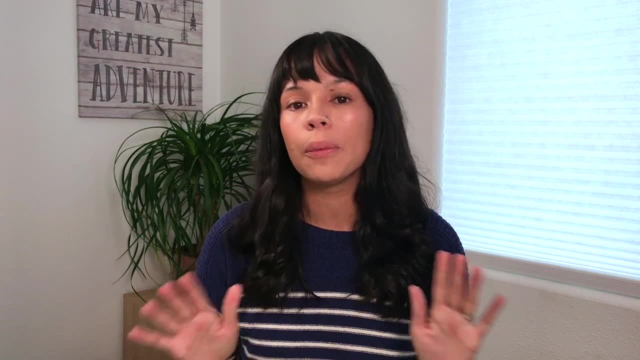 maybe one or two of these per day. I don't do entire exercises every single day. Don't look at this book and think, oh my gosh, how am I going to do these exercises in one day? That's not really that possible. Even in the suggestions to teachers section it does go over that. 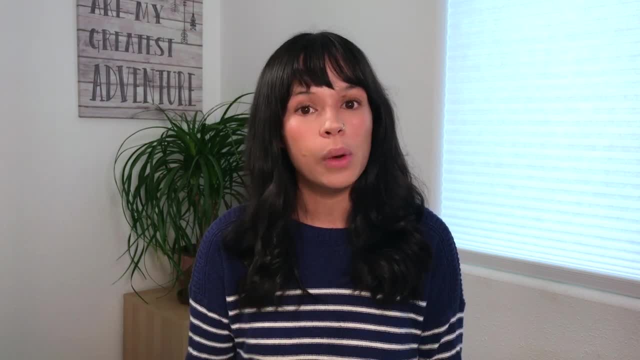 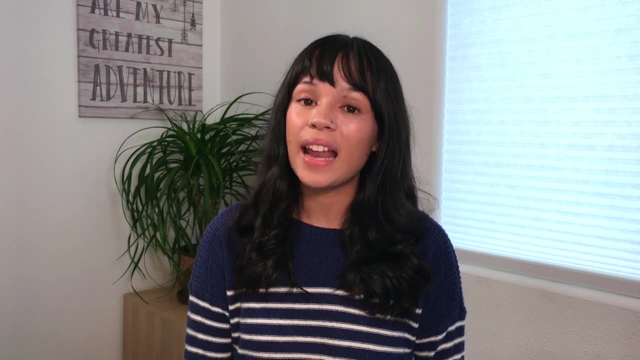 But so how we do this is we do one or two a day, So I'll read one of the sentences. my daughter will do her best to write it on her own and she has been getting better, so that's really cool. But then I will write underneath how it should be written correctly. 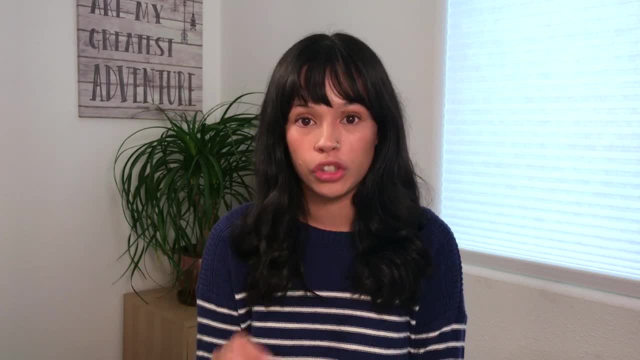 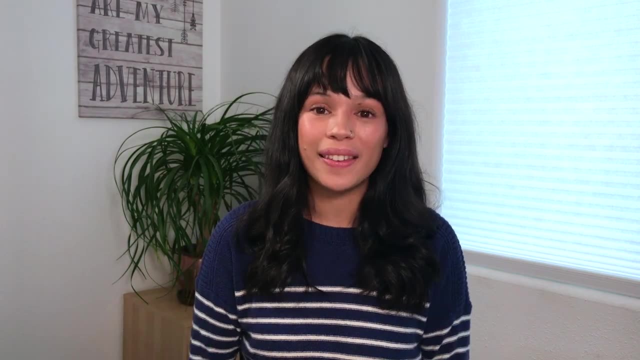 and then she does copywork, copying the exact way it should be written. So that's just how I've been doing it. This is the easiest way for me to correct what she has already done, And my daughter actually finds this kind of challenge really exciting. So 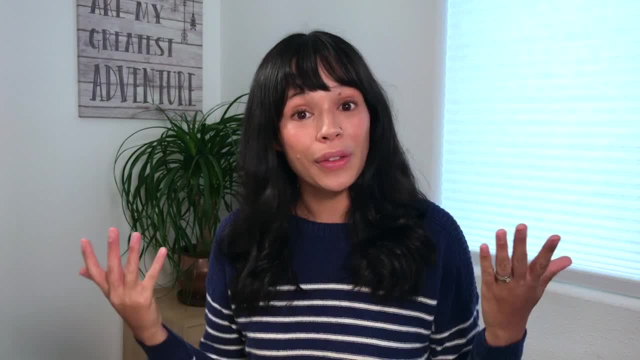 that's been motivating her to do better and better each time. Along with all these challenges, there are a lot of challenges that she has to deal with. For example, there are a lot of challenges that she has to deal with. There are also things like reading. 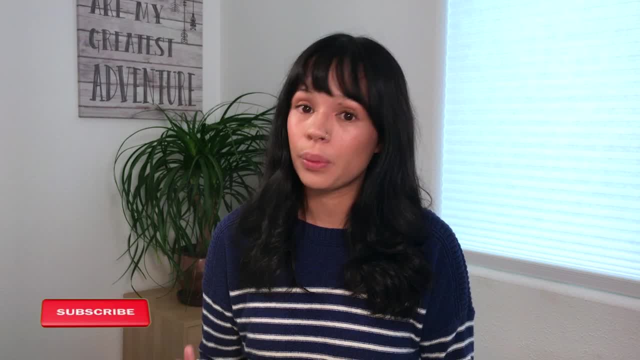 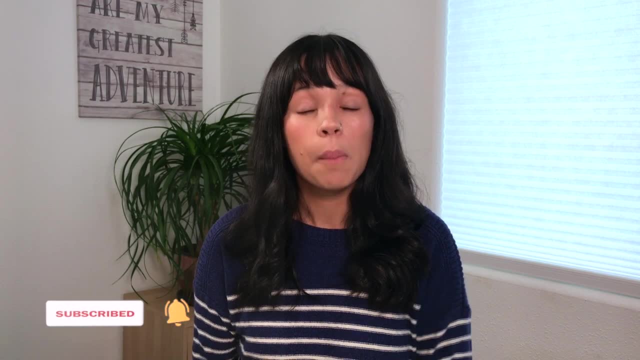 passages. So these start pretty short and your child is expected to read them aloud. And then there are also questions in which your child responds to the readings based on these questions, but doing so in writing. All of these different passages and questions do increase in. 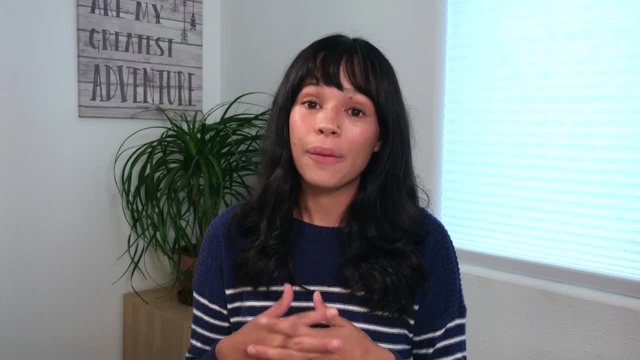 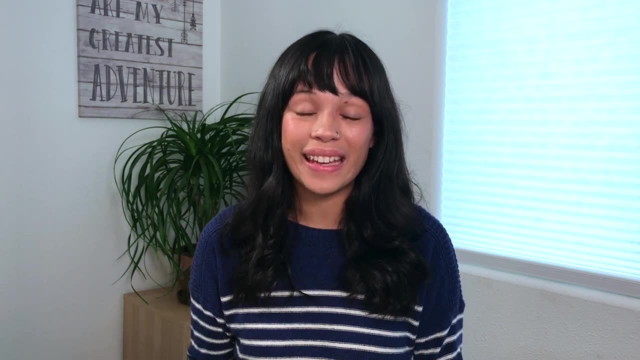 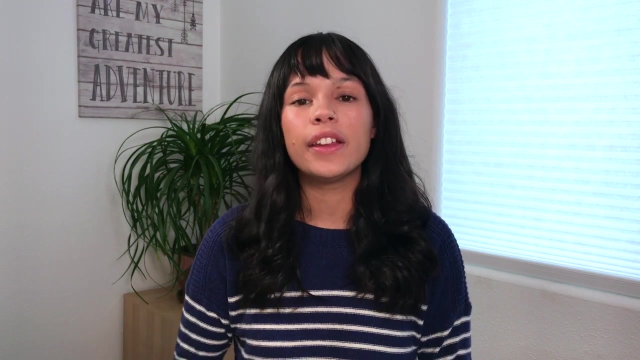 difficulty as the book goes on, And so far my second grader really hasn't had too much trouble with them. I think they're the right level of challenging for her. There are also kind of fun things like picture study, in which you can see different pictures done by great artists and then 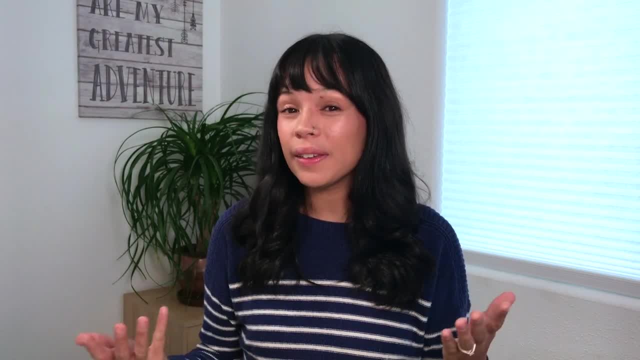 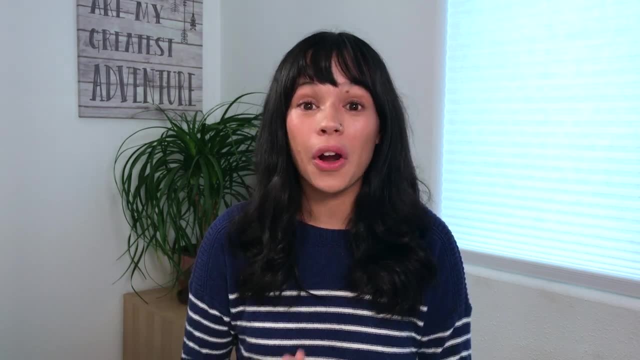 you react to them. There are also questions in the book that help get a conversation going about what they're seeing in the different pictures And, like I mentioned earlier, there are letter writing exercises, which I think is really cool, So I'm excited to get to those a little later especially. 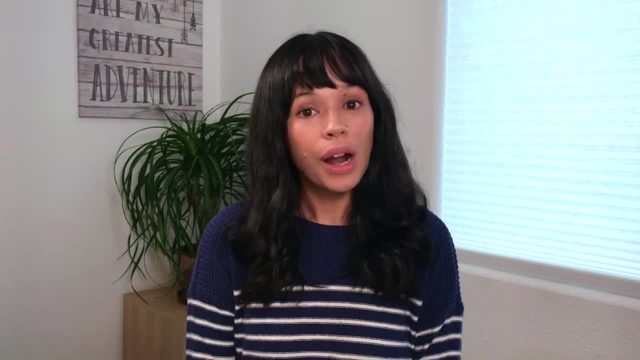 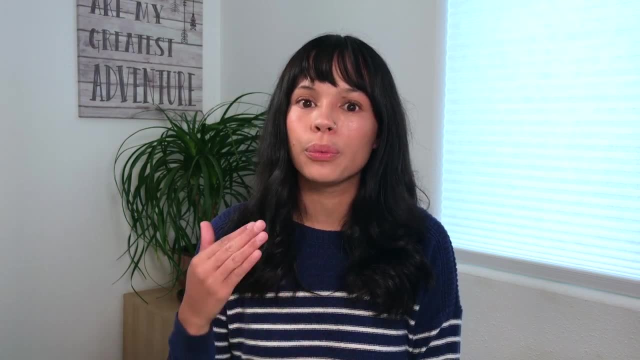 when my daughter is a little more advanced at writing. Primary Language Lessons is designed for second and third graders, And I've actually had this curriculum for a little over a year now, so I was really looking forward to when my daughter was in second grade, so I could finally